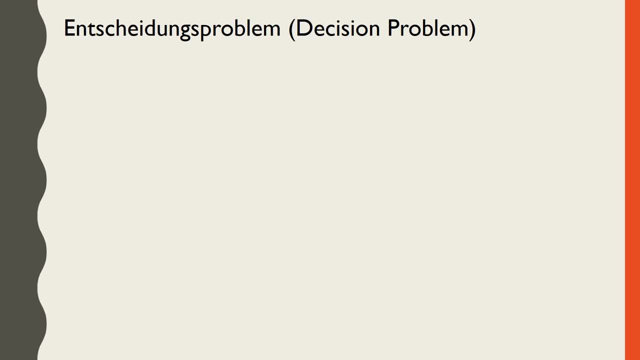 or decision problem. The decision problem is fundamental to logic. After having been around for some time, the problem was formalized by David Hilbert in 1928.. The decision problem is concerned with the validity of propositions. It rains when it is raining is true, for example. 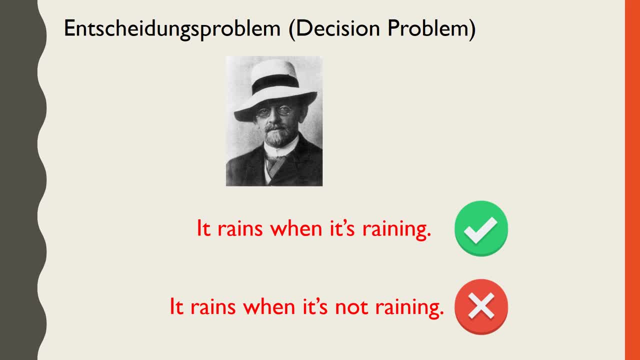 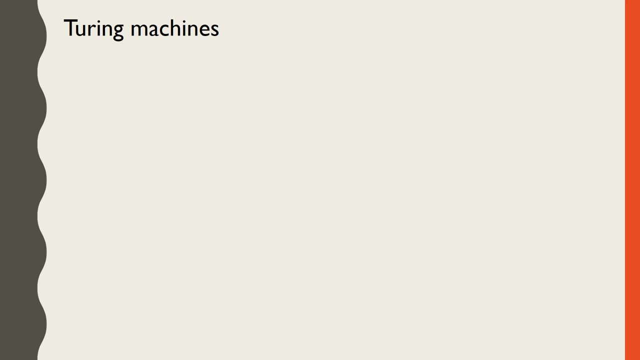 and it rains when it is not raining is false. Specifically, Turing was interested in the question: what is computable? The machine developed by Turing can mathematically describe any operation any modern computer can perform just by following a few simple rules. In fact, 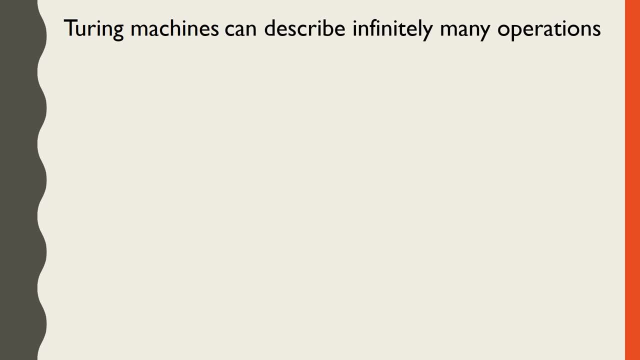 it's capable of describing infinitely many operations, though not every conceivable operation is possible on a Turing machine. Turing machines find applications in mathematics and computer science as powerful yet simple explanatory tools. Let's look at the basic parts of a Turing machine. One of the key components 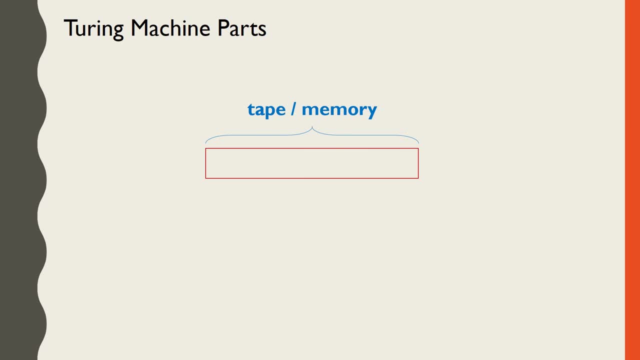 is a strip of tape called the tape or memory. The tape is infinite in length and divided into an infinite number of cells. Each cell holds a character or symbol which can be read or overwritten by the machine's read-write head, The alphabet of characters that can 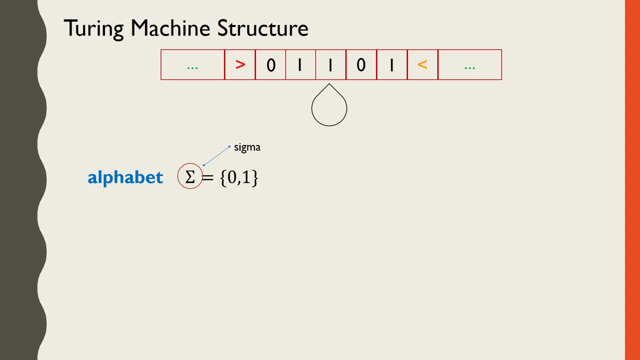 be represented by the machine is called the alphabet of characters. The alphabet of characters represented on the tape is given the name capital sigma. Our example machine in this lesson will use the characters 0 and 1.. 0 and 1,, then, are characters that are allowed to. 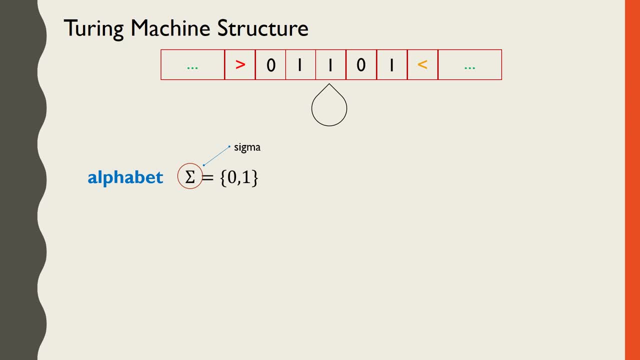 be written on the tape. There's another alphabet Turing machines use, which we call the tape alphabet and represent with capital gamma. It contains the 0 and 1 from sigma, as well as a few special symbols used in computations. These symbols mark the start position, the. 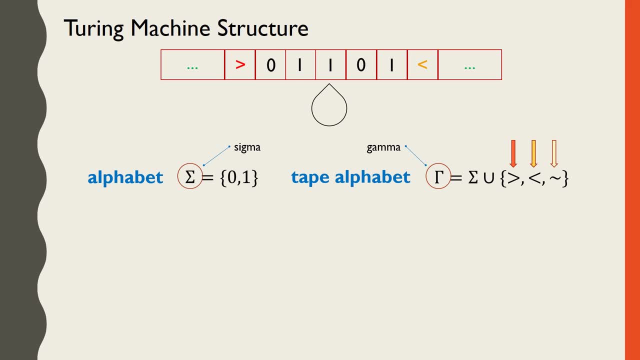 end position and a blank or unused cell. The portion of the tape enclosed by the start and end symbols is called the tape alphabet and represents with capital gamma. The tape is read-write head and is always positioned over exactly one cell and can read a symbol. 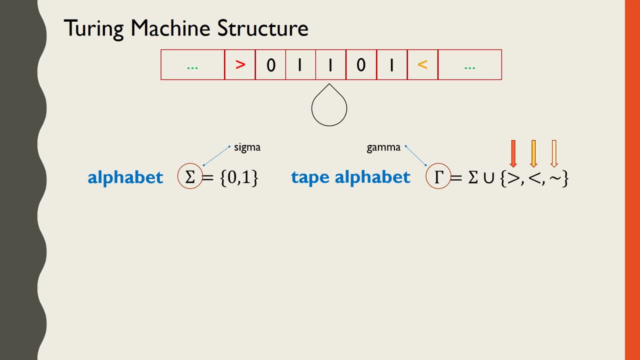 from that cell or write a new symbol in its place. The machine has the ability to move the tape one cell to the left or to the right at any time during operations in order to reposition the read-write head. It may also elect not to move at all during an operation. 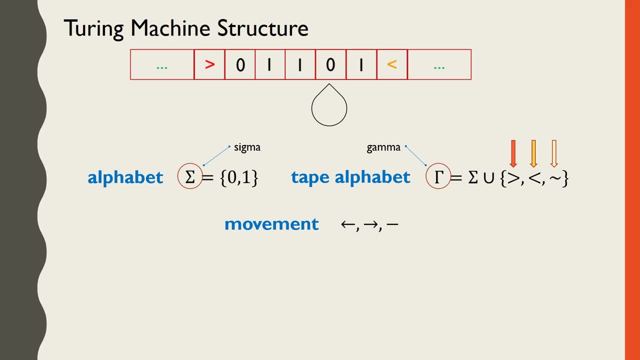 With this setup, the tape acts as both an input-output device and a storage medium for information. There's more that goes into the functioning of a Turing machine, like states and transition functions, which we'll explore in another video. The way Turing machines use this structure is the following: The input is written on.